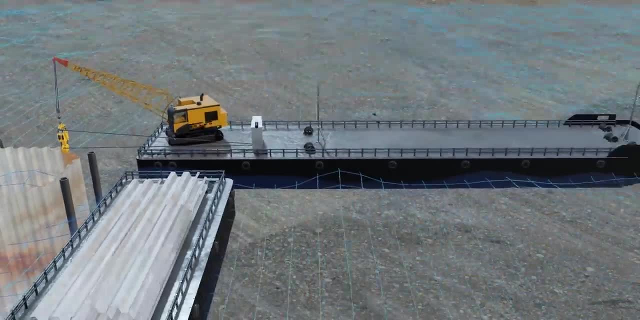 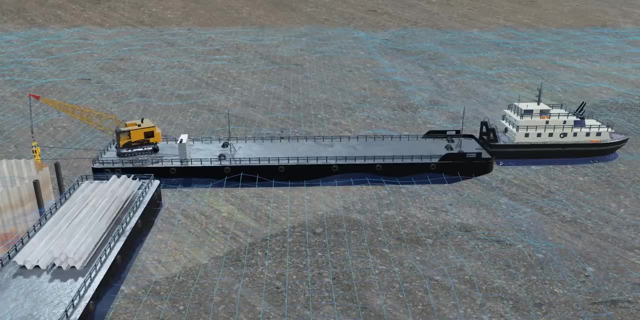 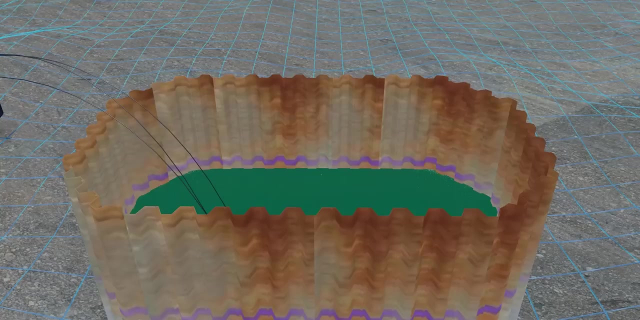 The purpose of these weights is to induce vibration in a machine. This flat surface-looking ship called a barge is employed to carry machinery and components that are required on the construction site. Now we're ready for the big phase of the construction project: pumping out the water from the cofferdam. However, before doing all this work, the engineers had a major assignment to do. Let's see what this was. before getting into the water pumping phase, The engineers of the project had to do a detailed geotechnical study of the soil on which the cofferdam was going to be constructed. They selected the land so that 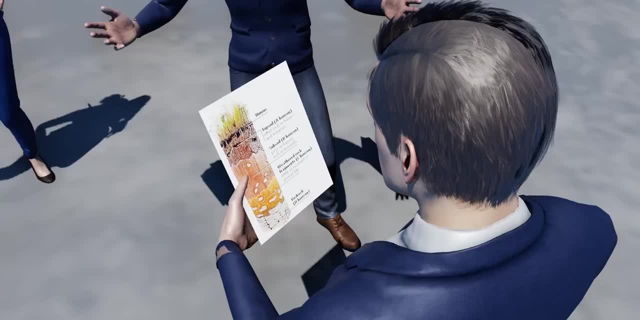 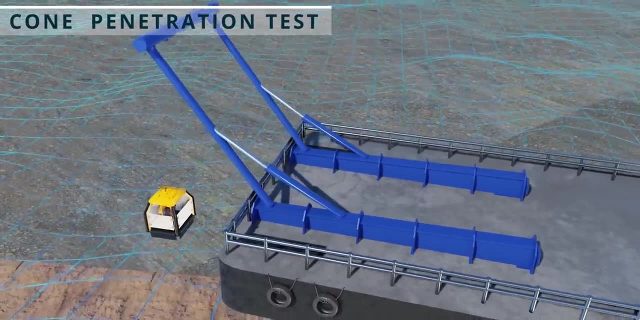 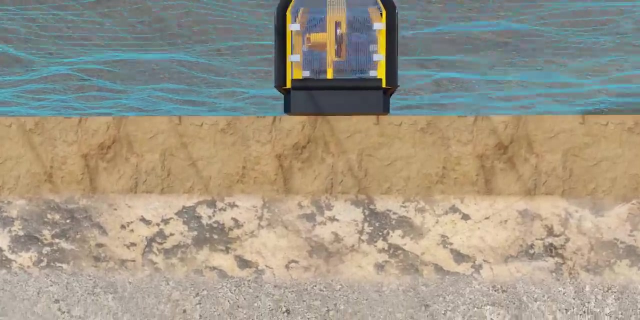 it would be able to carry the load of the permanent structure. The most commonly used test for measuring soil strength is an in-situ test called a cone penetration test. You can see how the cone penetration test device is kept on the ocean bed. The conical tip of the device penetrates in the 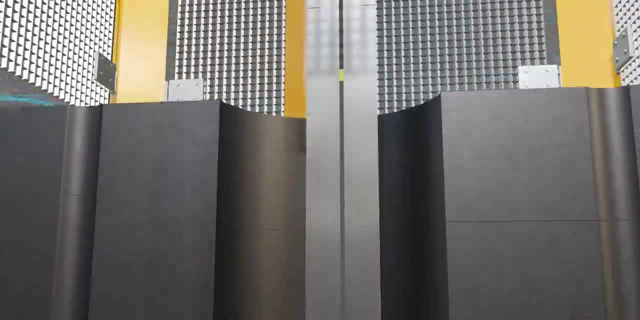 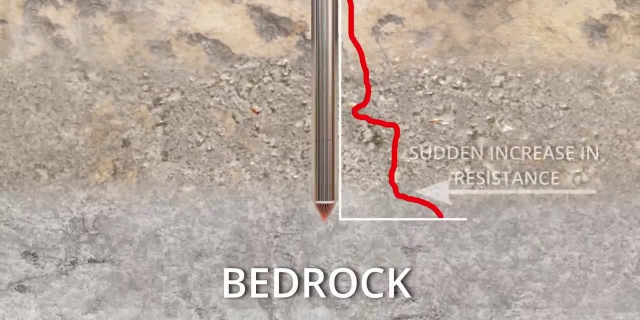 soil and sensors send back friction and soil pressure. The device is then used to measure the soil resistance values. They will continue the penetration till the point they reach the bedrock. You can see the sudden jump in the resistance value once the bedrock is reached. 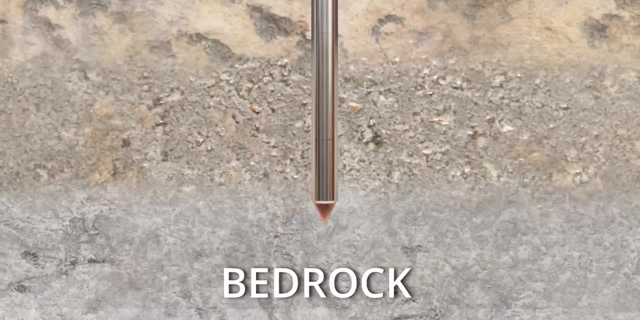 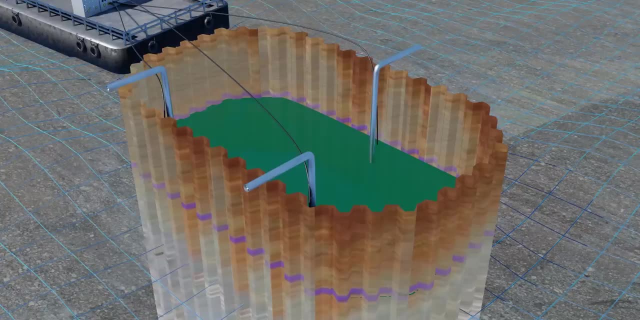 With the help of this handy test, the engineers know how deep the sheet piles must be driven. The sheet piles should reach the bedrock. Now let's jump back to the project and begin pumping water out. As the water level lowers, you'll notice water leakage between the sheet piles. 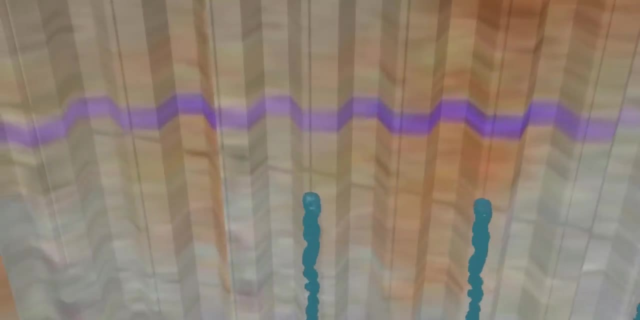 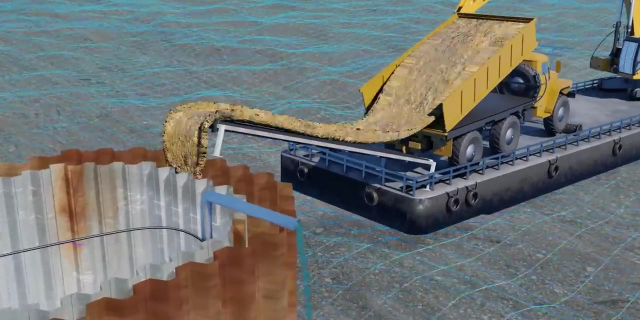 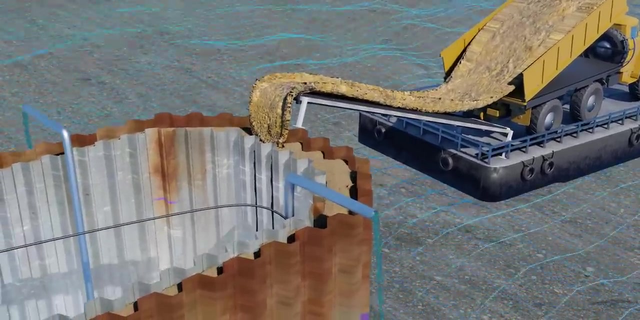 This is due to differential pressure of the water. Single-layer sheet piles are failing, so we need to double them. The space between these walls of sheet piles is generally filled with granular material such as sand, gravel or broken rock. This double-layered cofferdam will effectively resist water. 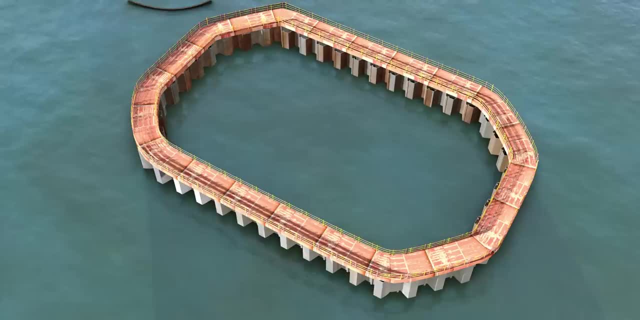 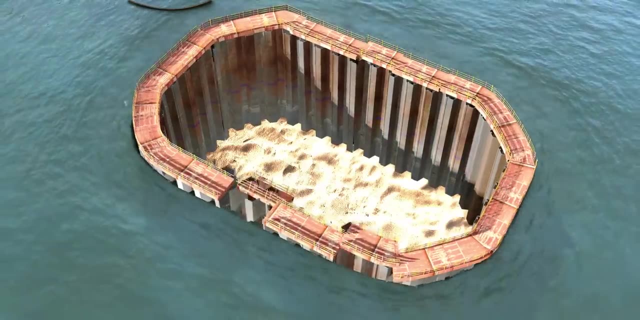 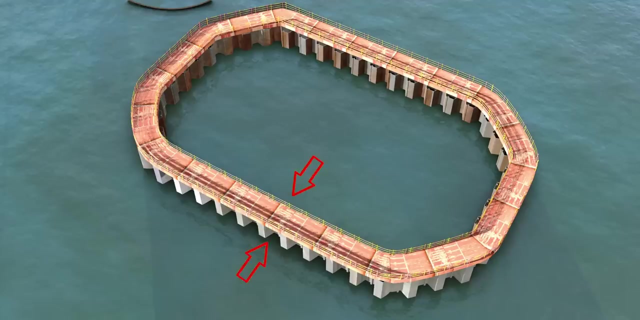 leakage between the sheets. Now let's remove all the water from the cofferdam. Luckily, there's no visible water leakage. Oh no, what happened? The entire cofferdam collapsed inward Earlier when the water was present on both sides. the force acting on the 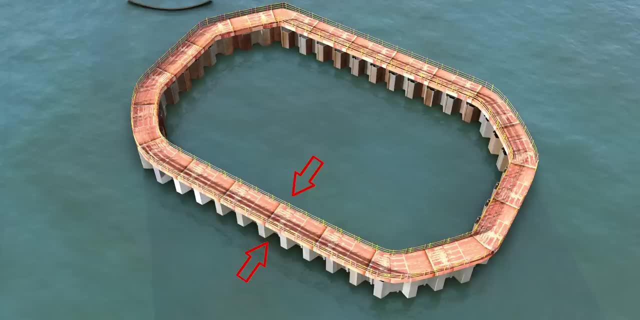 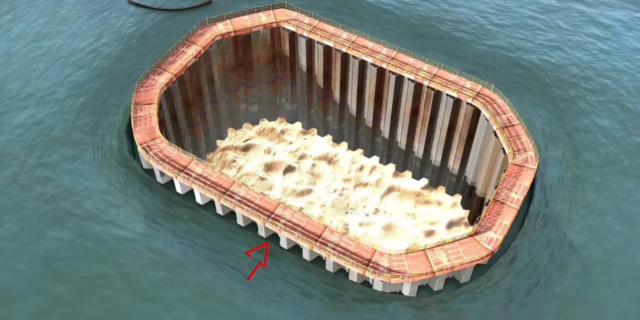 cofferdam due to the water pressure was being cancelled out. You can easily understand the reason for this. However, when the water from this volume disappears, there will be a huge inward force which destroys the cofferdam. The inward collapse of sheet piles can be. 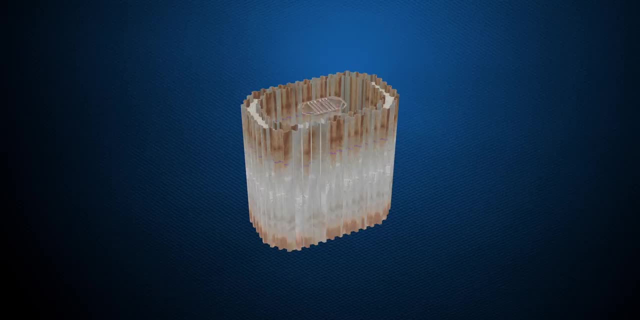 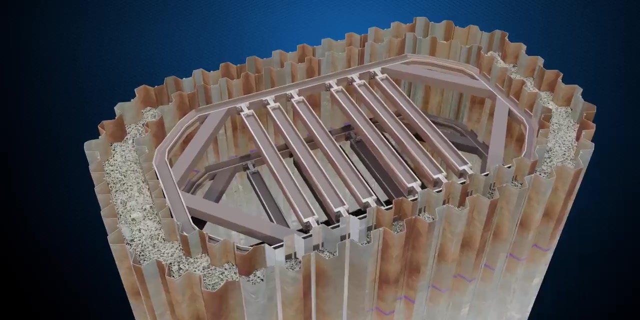 prevented by erecting a bracing frame structure by the side of the sheet piles. The bracing frame system comprises components like wales struts and braces. The connection between these wales and struts is bolted as illustrated here. 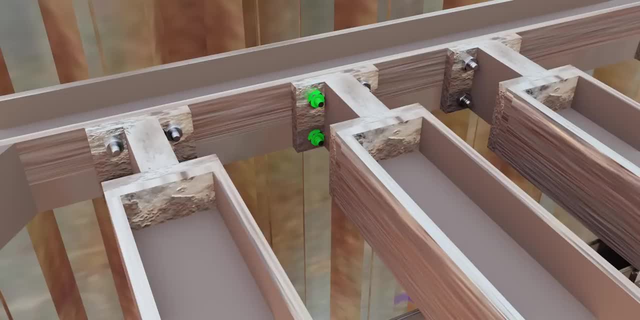 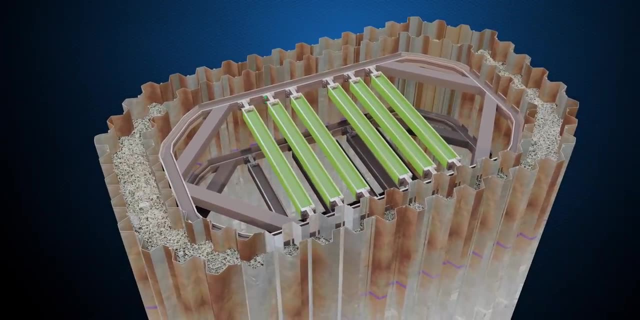 These horizontal members, called struts, provide lateral support which can resist inward movement to the cofferdam walls. The cofferdam is super strong now and it's reached the bedrock. Let's dry the water now. Can you predict what will happen now? 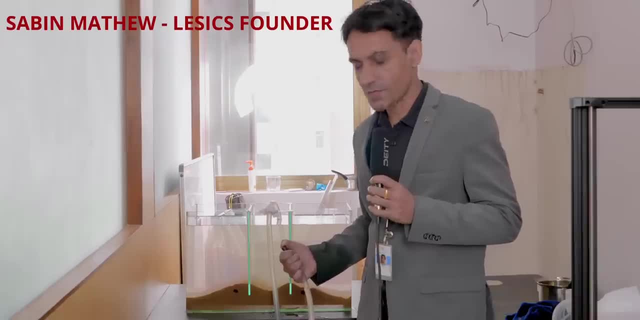 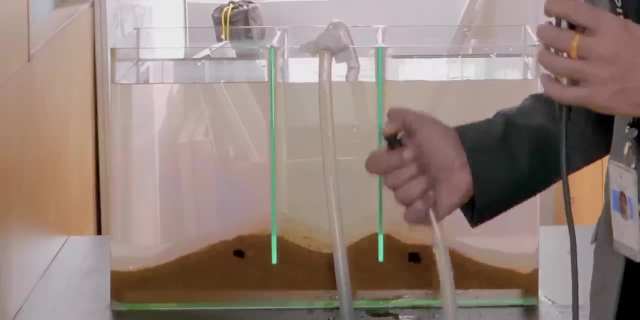 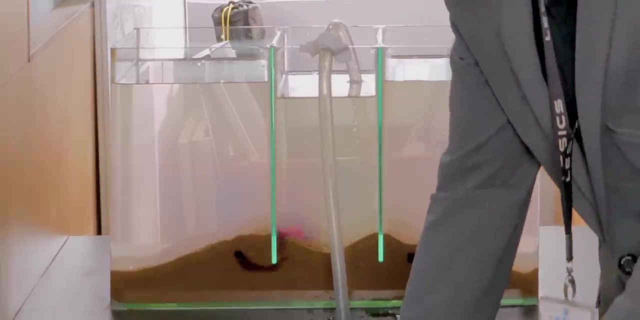 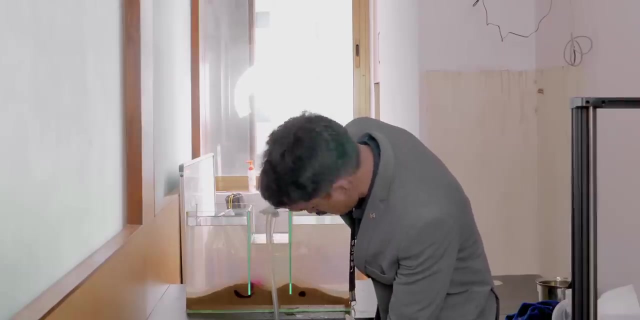 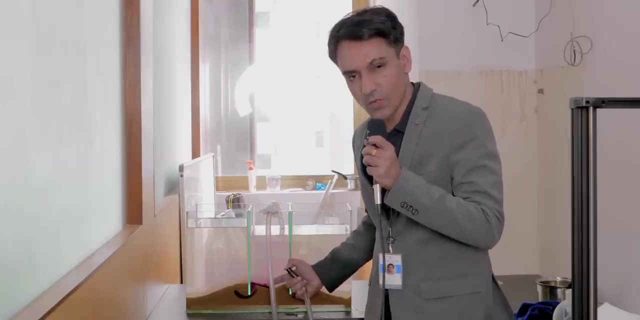 Here I have made a cofferdam- A small but cute cofferdam, isn't it? Let's see now what happens if I remove water from the cofferdam. I'm removing the water. Did you see that? A beautiful U-shape. The water particles are traveling like a U-shape below the 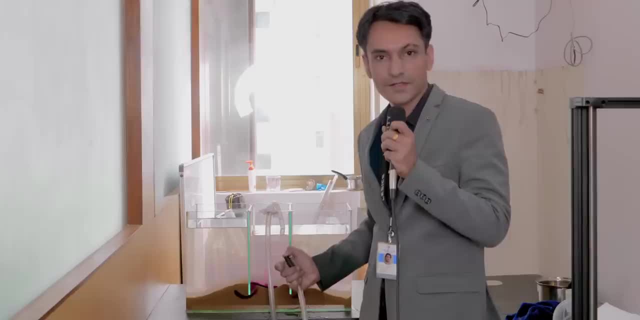 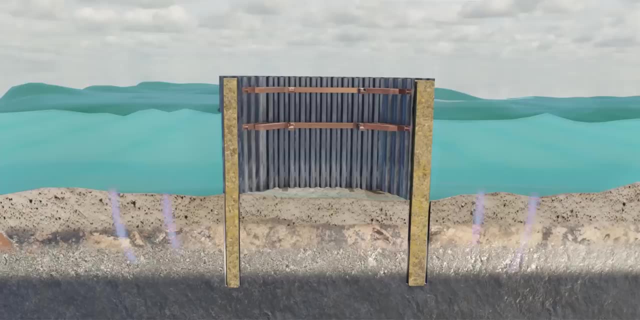 cofferdam. This is because of the water pressure differential. The same thing will happen inside our cofferdam as well when you remove water from that. Similar to the experiment, water seepage happens in our cofferdam also. The technique to prevent water seepage are difficult to accomplish. 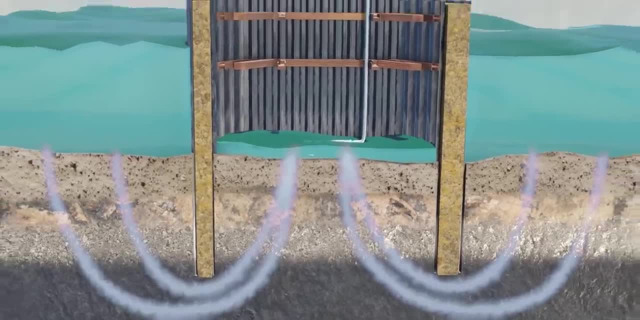 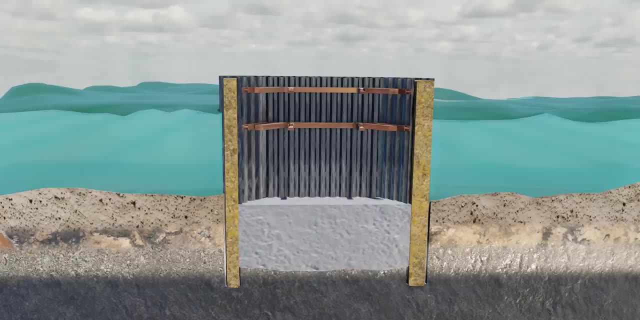 so let's pump this seepage water out continuously. If the soil above the hard strata is removed and concreting is done on the hard strata, our underwater project is half done. This is quite a piece of cake. This is called the concrete seal course technique. The concrete seal course will 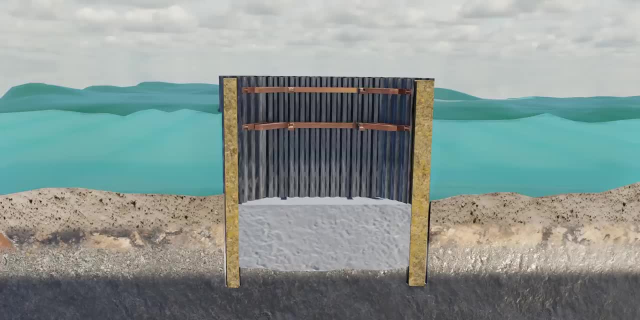 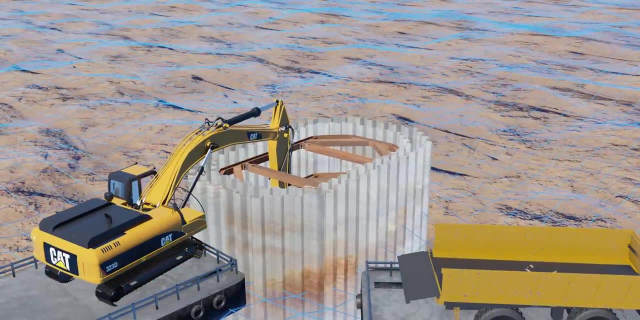 also act as a strong footing, preventing any water leakage. Let's see how this is done. The removal of the soil from the cofferdam is usually done using clamshell buckets. These buckets are operated by an excavator, Doesn't the operation of the clamshell bucket? 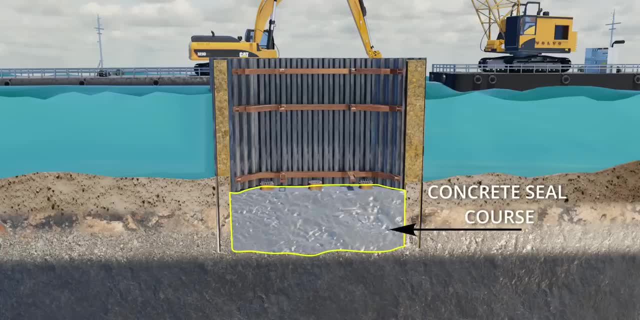 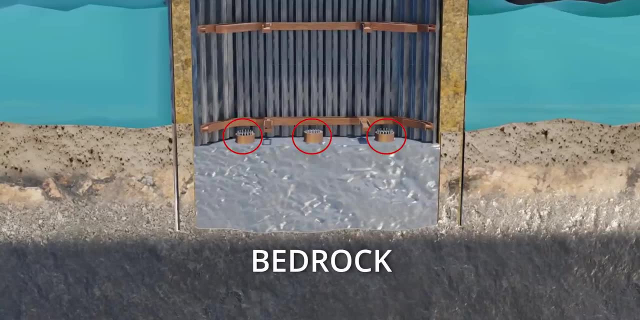 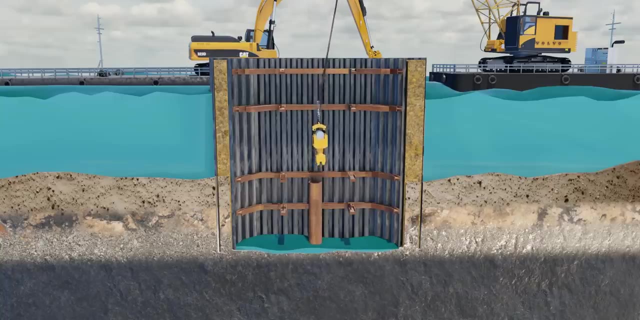 look pretty cool. You know the next stage: concrete seal course. To make sure the concrete seal course strongly with the bedrock, we need a few piles which penetrate into the bedrock. The vibrating hammer machine comes to help again. It pushes a few hollow steel pipes into the bedrock. The hard. 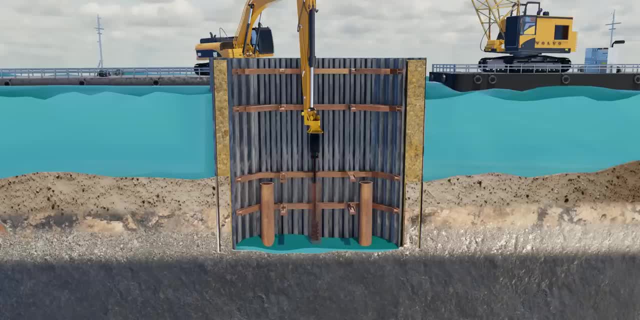 rock within this cylinder is removed with the help of an auger machine. Now it's time to place reinforcement bars into the cavity and pour concrete. Once the piles are ready, we can build the concrete seal course above, Since seepage water is present on this base- always the seal. 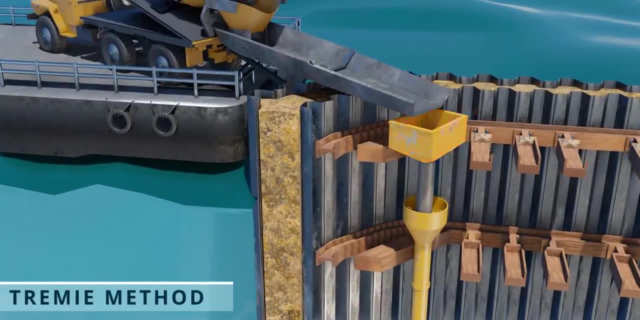 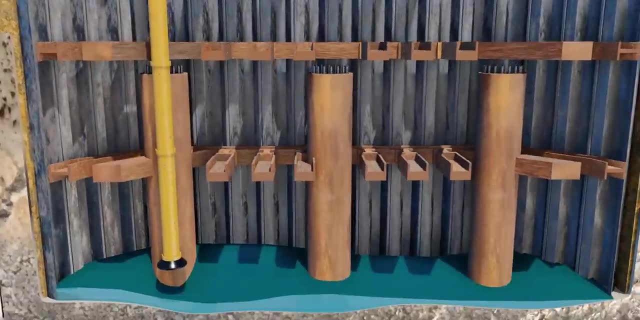 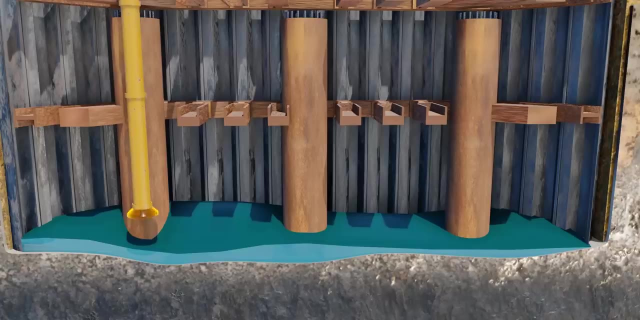 course concreting is carried out using the Tremi method. This includes a hopper bucket and a long segmented pipe. Specialized cement with high workability is used to concrete the floor. A thick plug is installed at the bottom of the Tremi pipe to prevent water from getting inside. 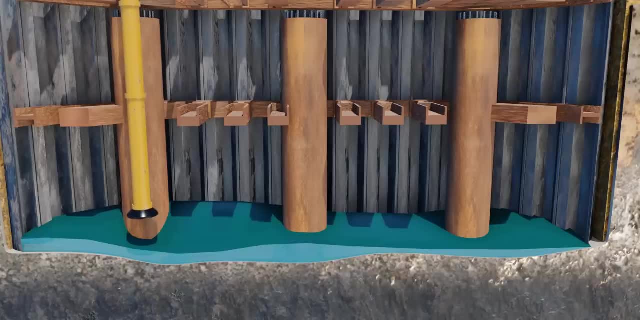 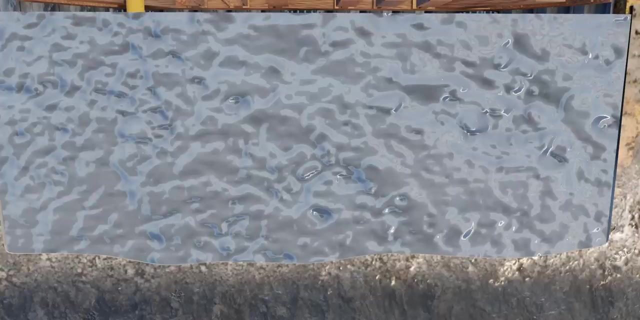 the pipe. After some time, this pipe is lifted with a jerk, causing concrete to pour down and the bottom plug to be removed. During this process, the discharge end of the Tremi pipe is continuously kept submerged in the concrete, so that the concrete which is getting 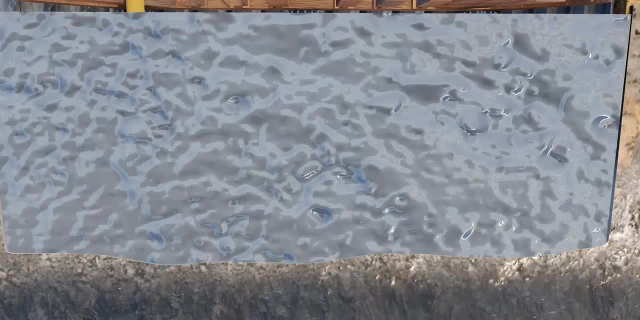 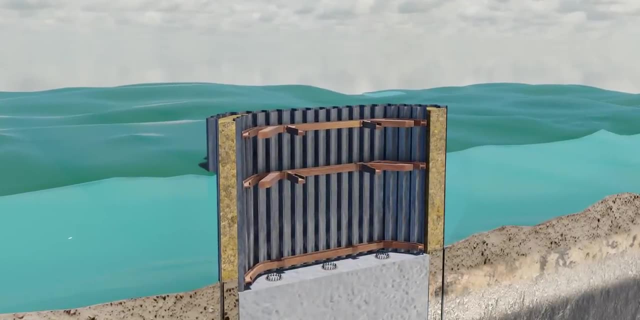 poured is less likely to mix with the surrounding seepage water. Now that the concrete seal course is ready, it's time to tackle the remaining construction work. The water seepage is efficiently blocked by this structure. Workers lay out the skeleton of high-quality reinforced 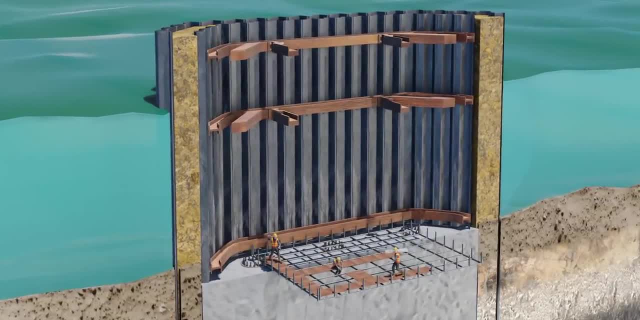 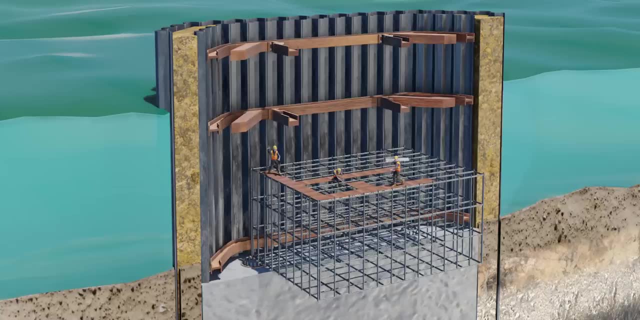 bars to construct the footing shaft of the bridge pier Because the bridge pier structure is going to remain in the water. engineers ensure that the bridge pier structure is going to remain in the water. This means that the materials to be used in the construction are of the best quality. 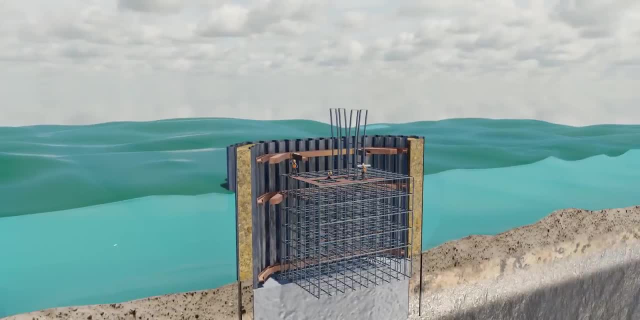 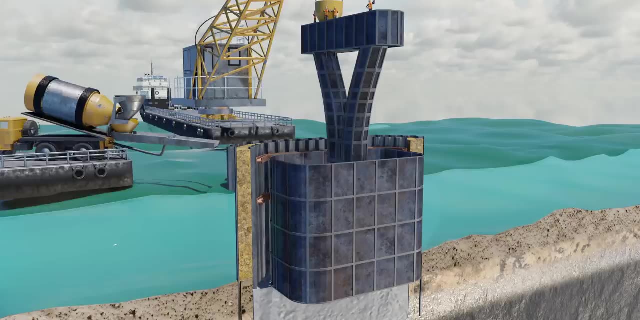 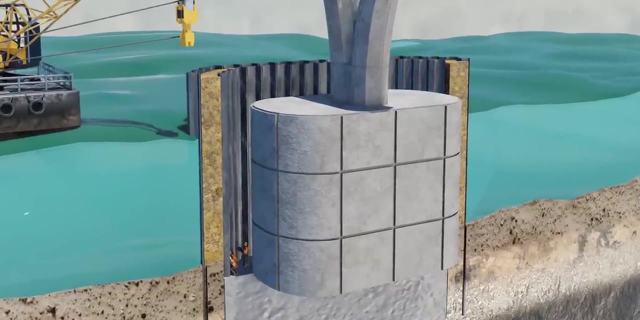 They must successfully bear the water pressure as well as the load of the bridge. As the skeleton of the bridge pier keeps on progressing, arrangements are made to pour concrete in the structure. Once concrete is completely poured into the skeleton, this structure is kept undisturbed to gain strength. Usually, a bridge pier takes 14 to 28. 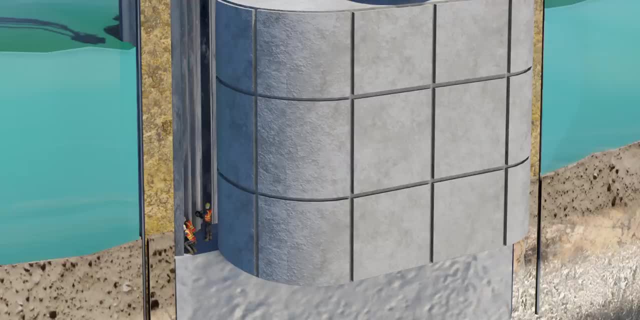 days to gain complete strength. Once the bridge pier gains enough strength, the dam is no longer in use and is an eyesore, so the engineers remove it. However, removing the cofferdam below the level of the concrete seal course can affect the strength of the whole. 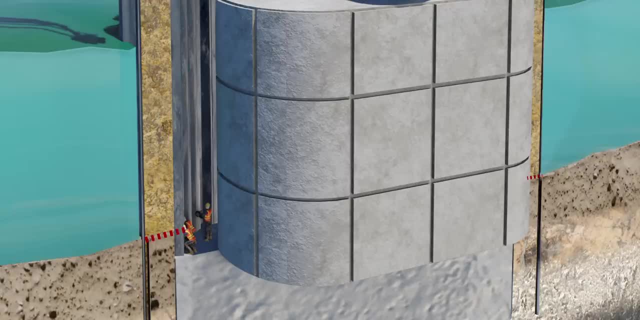 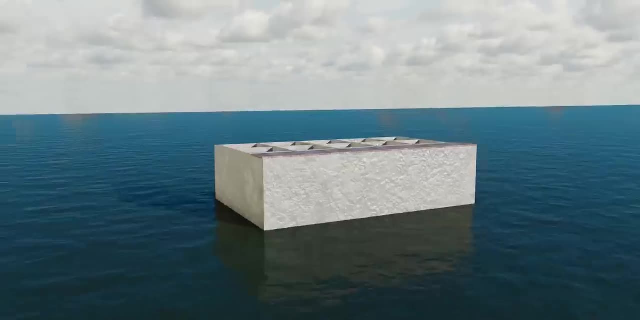 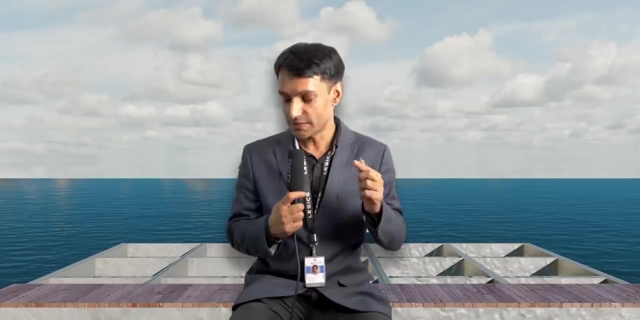 structure. As a result, engineers cut the sheet piles at this level. Here it is. This strong bridge pier is ready to support a heavy bridge. I hope you enjoyed the video on underwater construction technology using cofferdams, But this is a different kind of bridge pier.